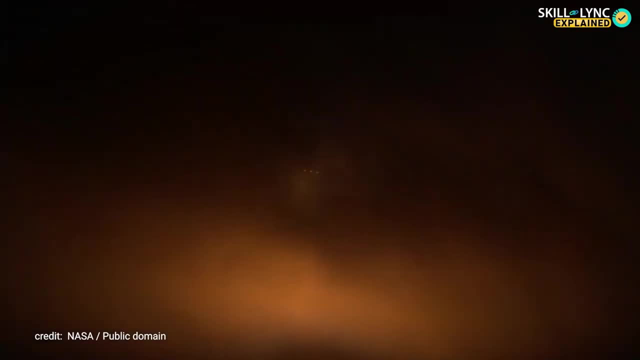 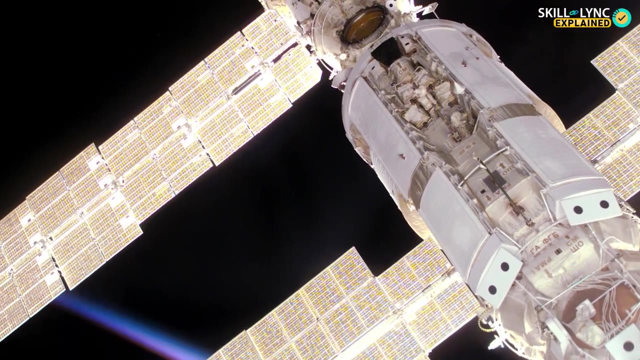 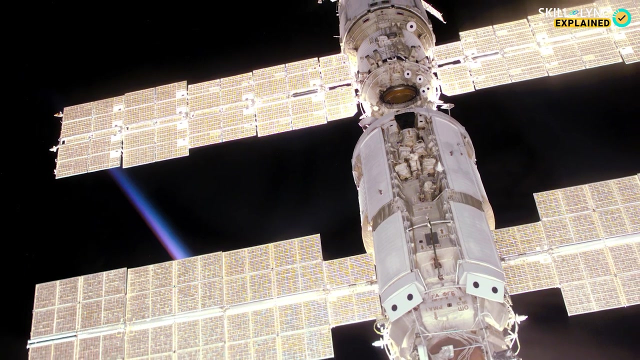 but even those fail to provide energy for large distances. The only option is the use of energy from our star, the sun. By installing solar panels into satellites and space probes, the supply of energy can be ensured. But again we face a problem here. Solar energy can be an excellent power source for the inner solar system, But 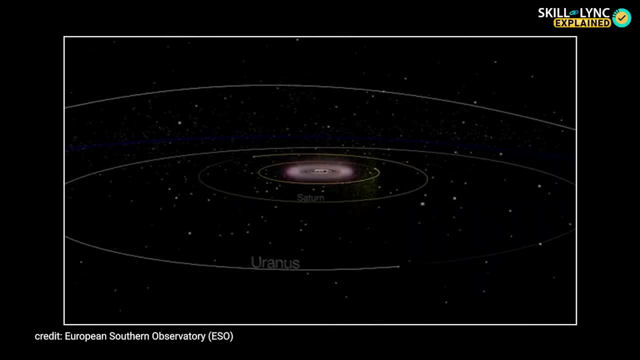 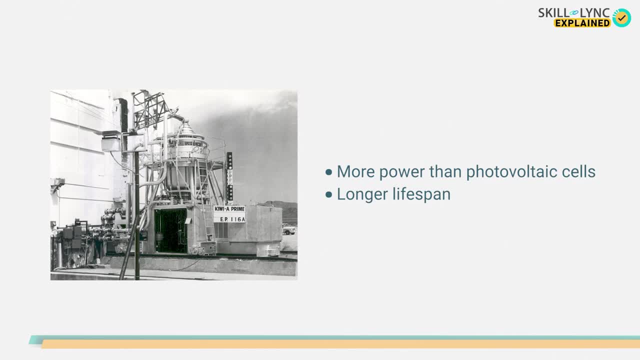 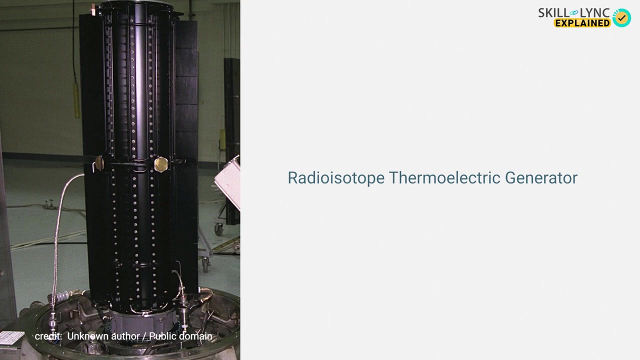 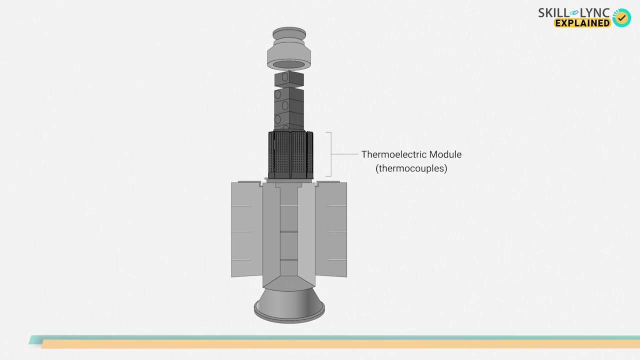 space exploration. Nuclear power is an excellent energy source for long-distance space missions, because nuclear energy not only provides way more power than photovoltaic cells, but it also has a much longer lifespan. Nuclear power is utilized for space flights in RTG's or radioisotope thermoelectric generators. RTG's are devices that use an array of thermocouples. to convert the heat from the gas stoves thermos and� the neutron degree thermos intouation. It waist-łbym 발생ence similar to that, episodes around那个 thermal pasteurization device fromến heat has been activated in這個是. 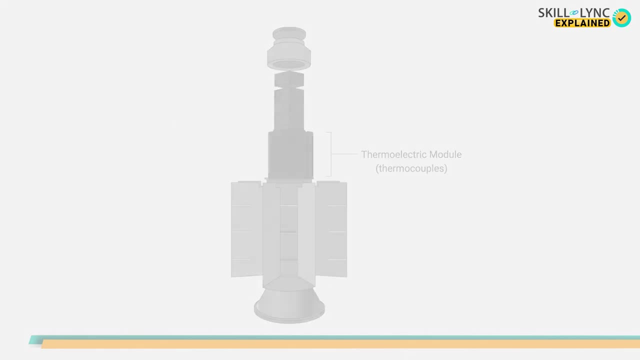 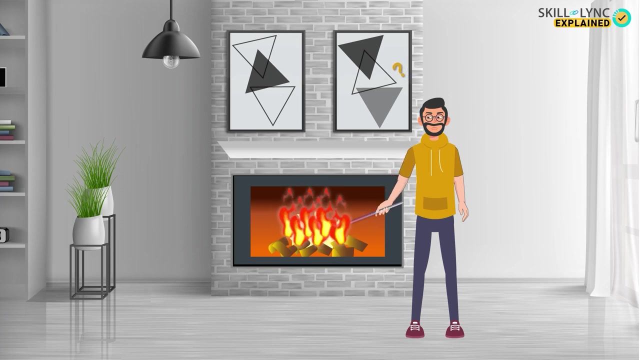 decay of radioactive material into electricity. We all know that if we put a metal rod near fire, it will get hot rapidly. But there is one more phenomenon happening there. That phenomenon is the Seebeck effect that is used in thermoelectric generators. 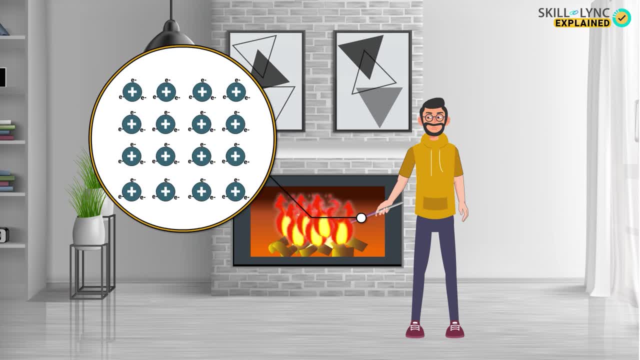 We know that in metals heat is conducted easily because the electrons are free to move, But those electrons can also carry charge. Thus, if a metal rod is placed in a temperature gradient, then an electric potential will be developed between the two ends, resulting in the Seebeck effect. 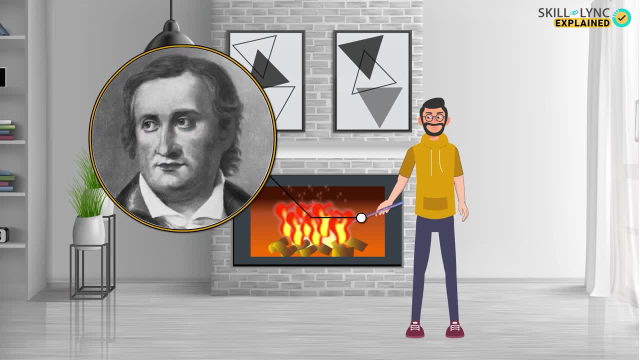 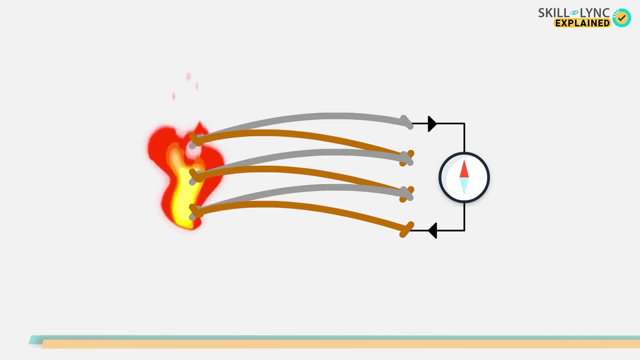 This effect is named after physicist Thomas Johann Seebeck. He observed the deflection of a compass magnet when a circuit made of two dissimilar metals had junctions at different temperatures. The reason behind this was that the movement of electrons was different in different metals. 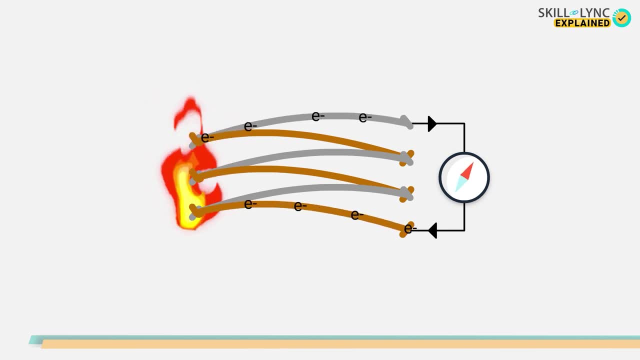 This created a potential difference that caused electric current in the circuit and therefore a magnetic field around the wires that deflected the compass. The voltage produced, called the Seebeck voltage, is directly proportional to the temperature difference between the two junctions. 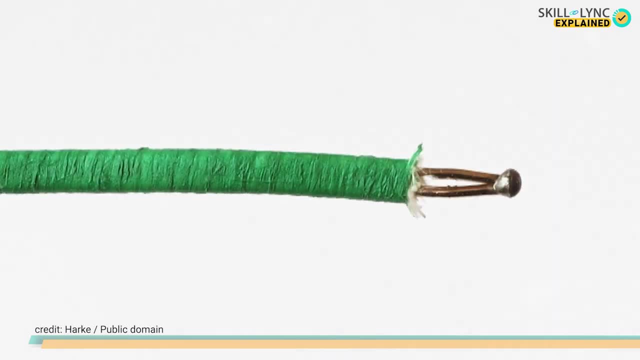 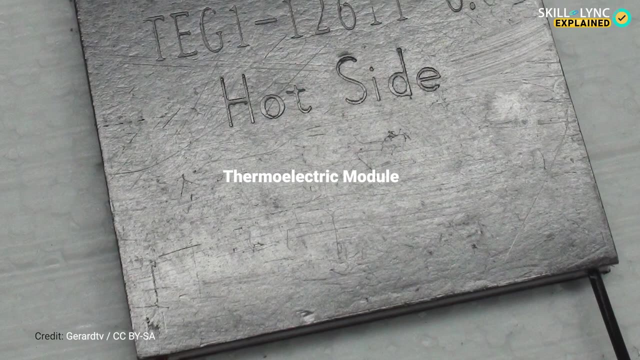 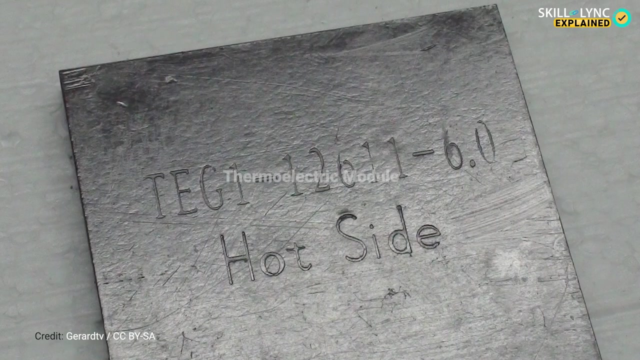 The device that produces a temperature-dependent voltage as a result of the Seebeck effect is called a thermocouple. A radioisotope electric generator needs a larger multiple. Therefore, a large number of thermocouples are connected in series to produce high voltage. 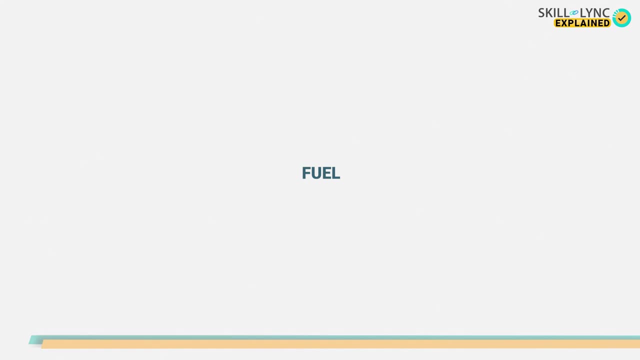 Moreover, the radioactive element used as a fuel in RTGs must have a long enough half-life so that it releases energy for a considerable amount of time. In addition, the radiation from the radioactive element should be easily absorbed and transformed into thermal radiation To comply with all these needs. 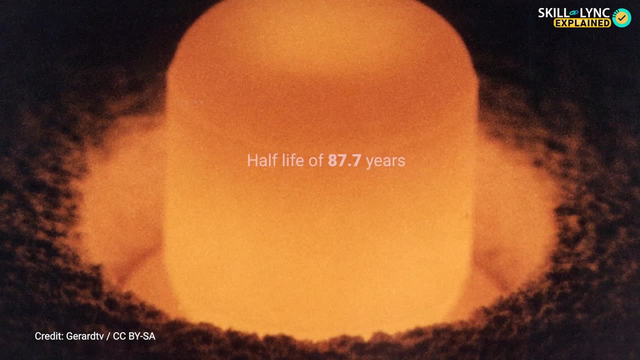 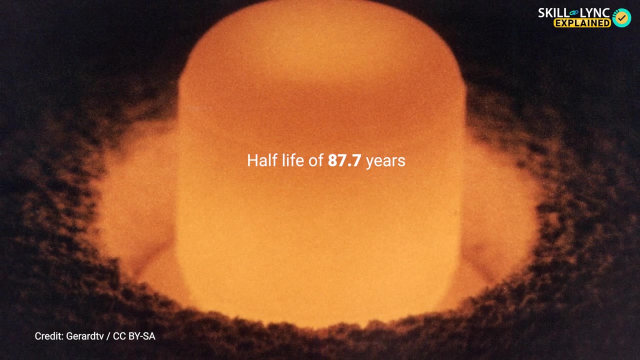 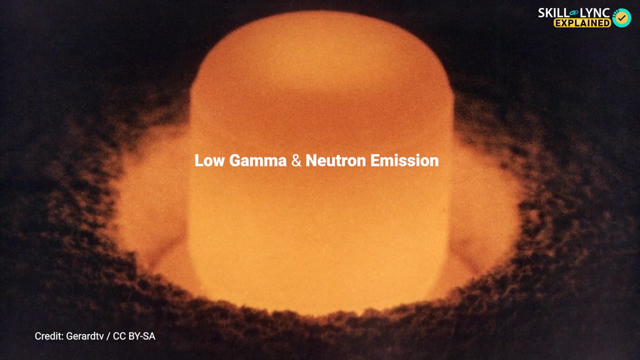 Plutonium-238 is used as a fuel. Plutonium-238 has a half-life of 87.7 years, meaning it takes that long for its heat output to reduce to half. Also, it has the lowest shielding requirements because of very low gamma and neutron radiation. 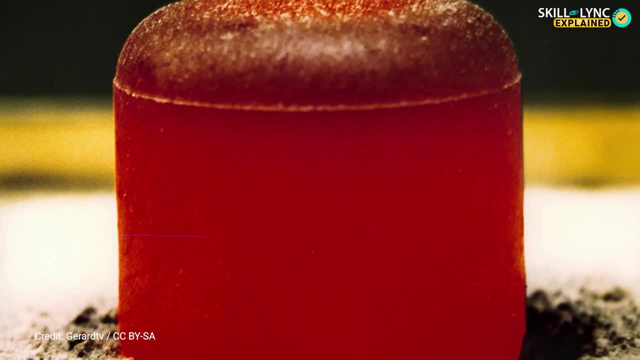 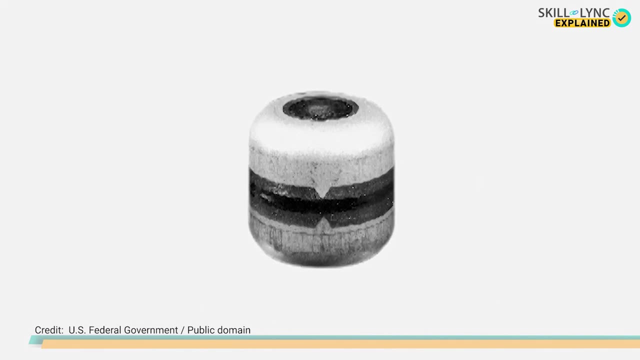 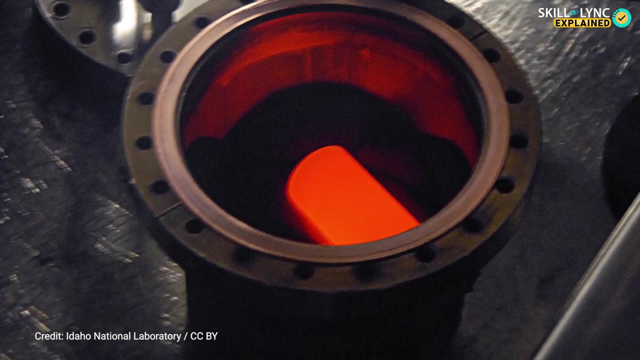 So Plutonium is used in RTGs in the form of Plutonium Dioxide, To block the alpha particles generated by radiation. they are clad with iridium. This is then placed in a graphite shell and assembled into a complete module. 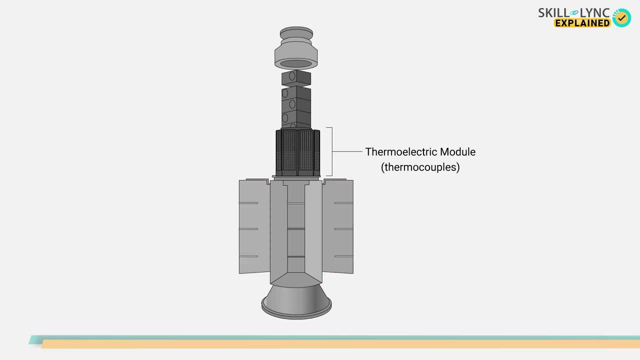 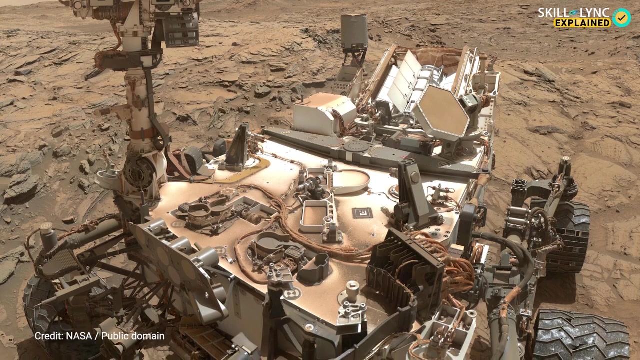 These modules, called general-purpose heat source modules, are then stacked together with thermocouples For dissipation of heat from the generator. radiator fins are provided. RTGs need no maintenance since they do not have any moving parts. They have been used in numerous space missions, including Curiosity Rover, Cassini and NASA's 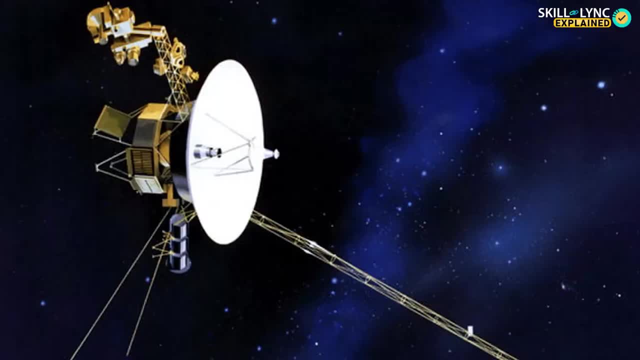 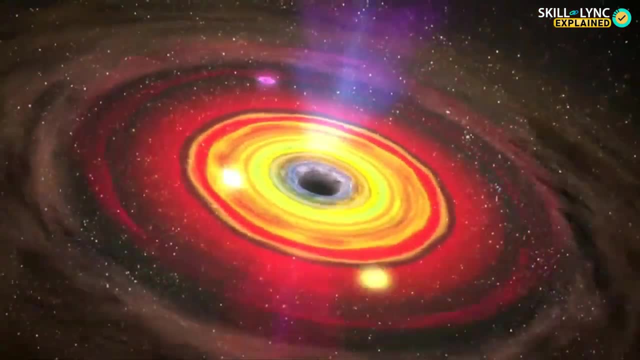 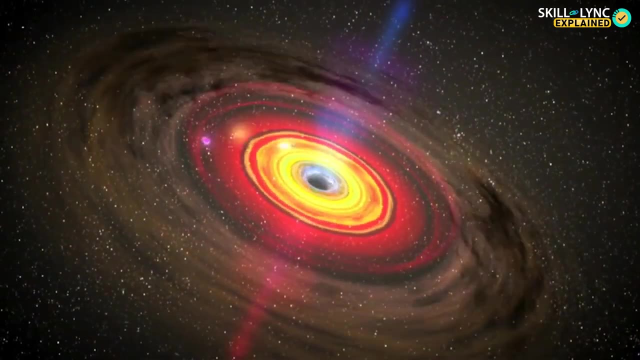 space shuttle: New Horizons, Voyager 1,, Voyager 2, and even in the Apollo program. So, guys, nuclear power has a wide range of scope for use in space. Maybe one day we will be closer to traveling into interstellar space when they use more. 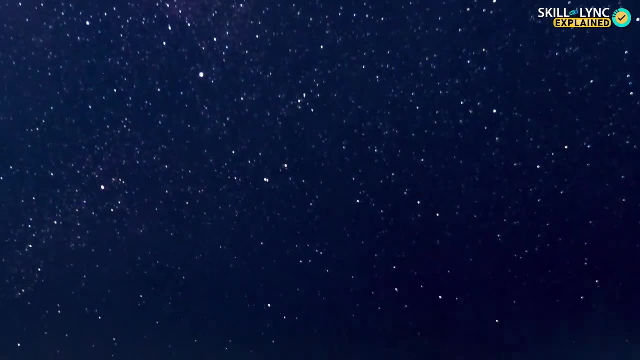 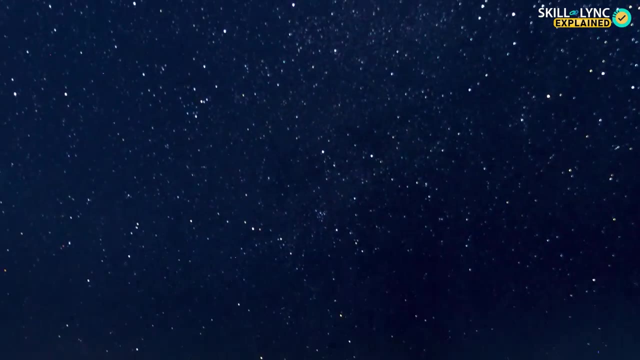 such advanced technology. But until that day comes, don't stop looking into that night sky for answers. Who knows, maybe it's not so empty after all. We'll see you next time on Skillink, and until then, bye. . .